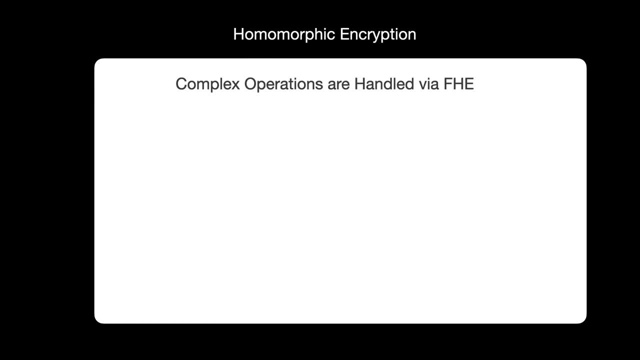 modeling services in more than one area of the world. A company- XYZ- offers services- machine learning, modeling services in more than one area of the world. A company, XYZ- offers services machine learning. you know, that's maybe something for another video. it's a little bit more complicated than this, but 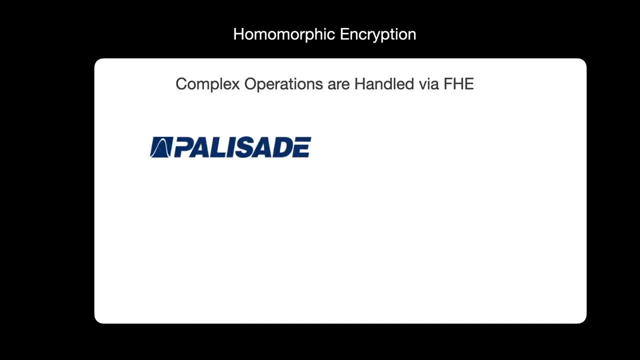 you know, there are some pioneers out there. for example, palisade has got some implementations out there that you can download. ibm has one, and one of the more popular ones is by microsoft, which is actually called seal, and there's a python version called pisil which you can go check out. 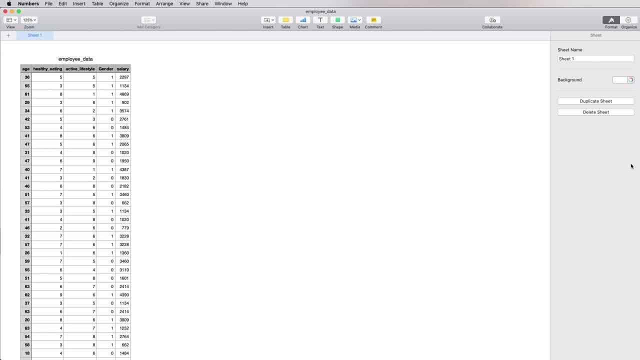 as well. there's a docker image for it that you can open. so when i really look at the example that we want to go through today, it's something very, very basic. what we're trying to do is we're trying to predict somebody's salary based on some numerical facts about them. so first we're going to be: 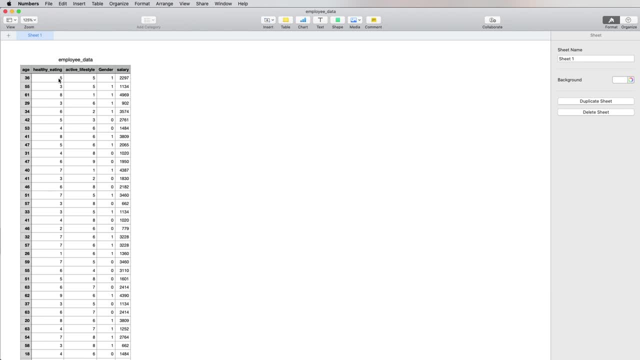 looking at their age. we'll be looking at their active lifestyle, to see whether they're active and whether or not they're eating healthy as well and as well as their gender. now, in reality, you'd be looking at a multitude of other variables, but just for the purpose of this, like i said, we're 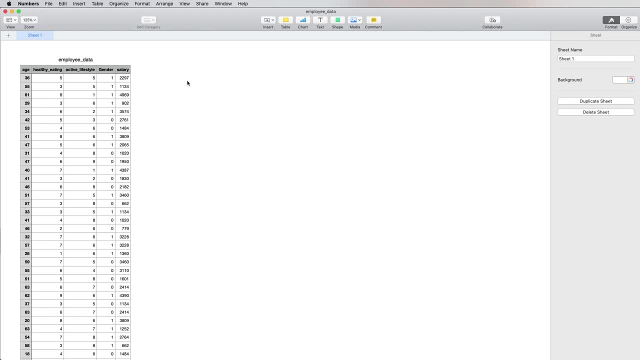 going to be building a toy model. these are the sort of the five data points that we have, and we'll be using four of them to do a prediction against salary. and, again for the purpose of keeping this very simple, we're going to be using a linear regression model that we're going to go ahead and build in python. so let's get started. 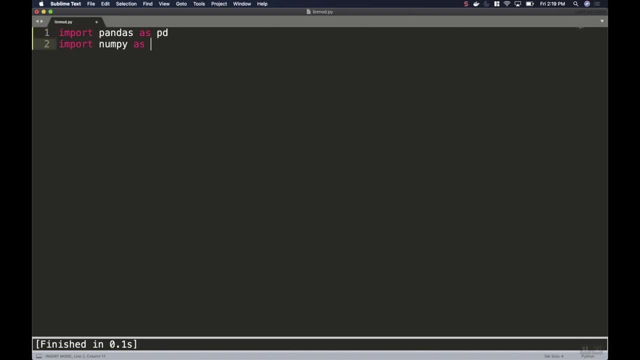 all right. so one of the first things we're going to do is we're going to go ahead and open up a new file called lin model. in lin model, i'm going to be importing a whole bunch of different dependencies from pandas, numpy, phe, more specifically the paler method, sklearn, and in sklearn we're going to be 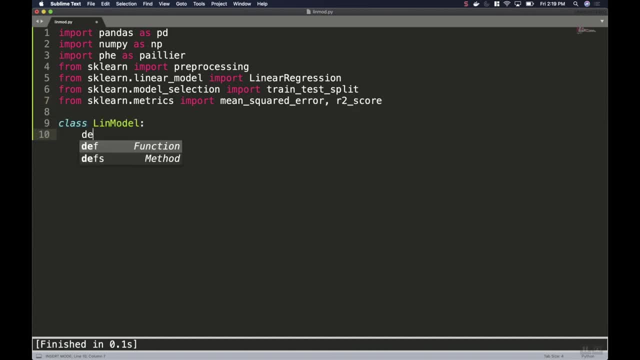 using the linear regression model, train test. split mean squared error and r squared. i'm going to go ahead and create a class called lin model and that's going to be my linear model. so get results in lin model. it's going to be my linear regression model and it's going to be my test and train. 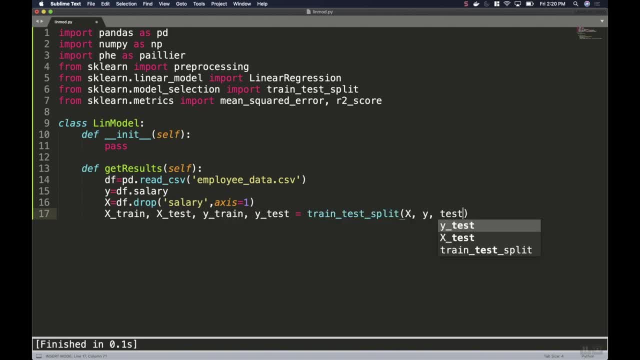 split, and then i'm going to go ahead and fit my test data against my linear model and then i'm going to go ahead and predict my train split, which you'll see coming up very soon as well, right here. once i have that, then i'm then i'm going to go ahead and look at a few different metrics, like 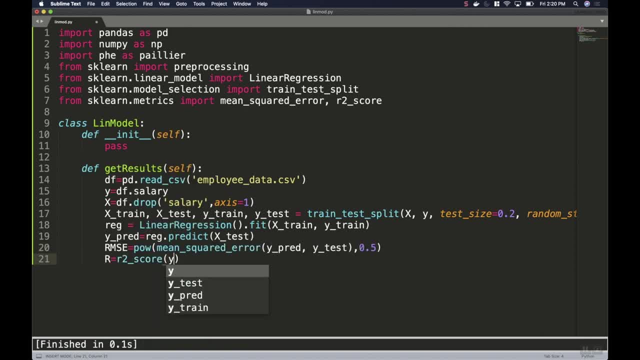 root mean squared error and as well as the r square- and just let you know, i looked at the r square is about point eight, four or so. and again, i'm not looking for perfection in this model, but model. It's just sort of a toy model. at this point, The more important thing is to get these. 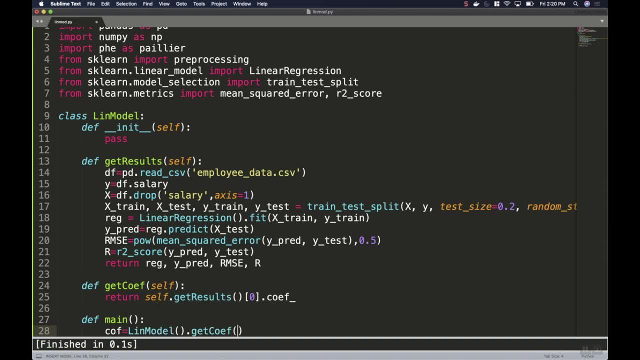 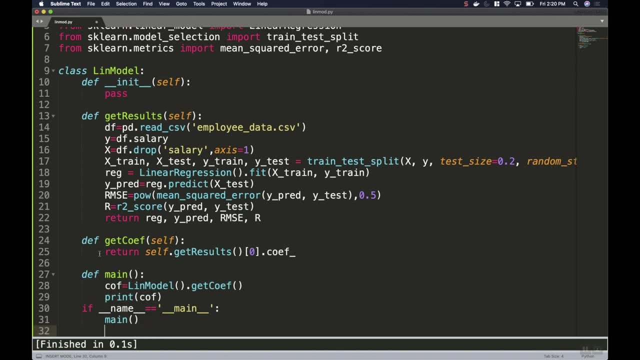 coefficients, or the weights of the actual regression model, And that's what I'm going to be using against my encrypted data. So very soon, in just a quick second, I'm going to go ahead and print these coefficients And these are the four coefficients that are going to correspond. 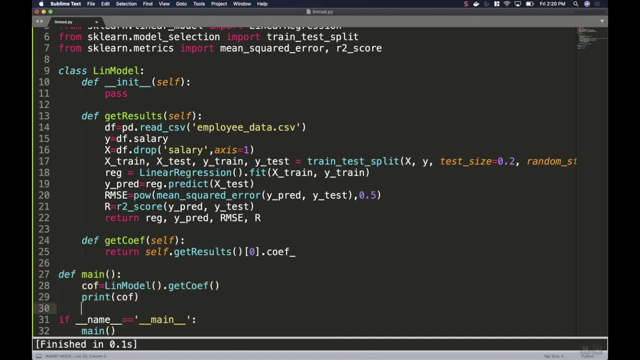 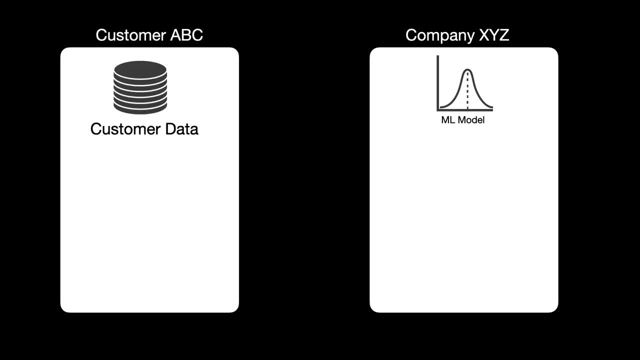 to my age, my healthy eating, my lifestyle, as well as the gender as well. So these coefficients are the ones I'm referring to as right here. All right, So that really completes my ML model, the one that the organization is going to be using, And we just created that. 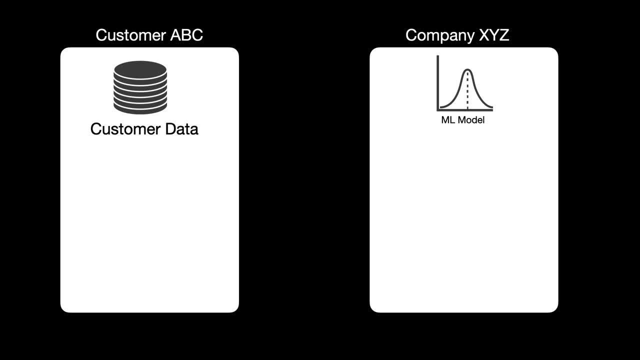 The next thing we're going to do is we're going to go ahead and create some simulated data for the customer. Then we're going to create an instance of a public and private key And we're going to encrypt this data with a public key. So let's go ahead and do that next. Okay, First. 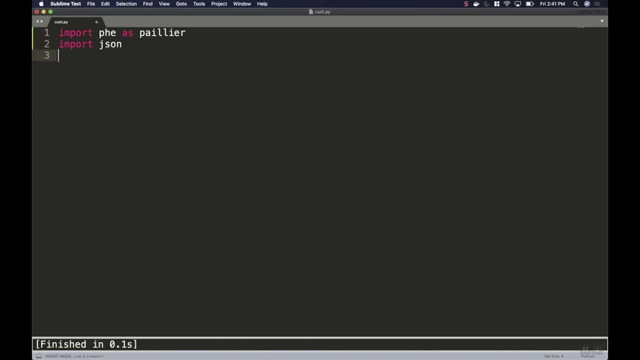 we're going to create another file, called customerpy in this case, and this is going to be the customer's file. In here we're going to create a method called store keys And in there we're going to create an instance of public and private keys generated by the paler. 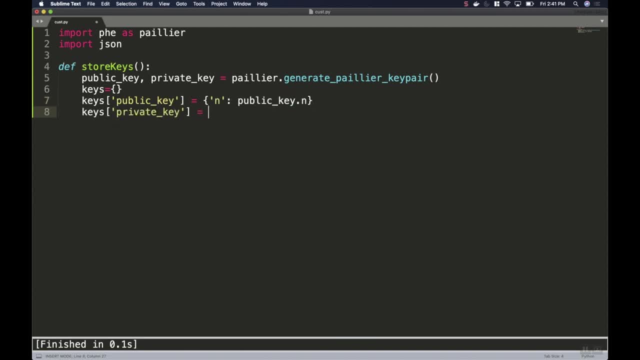 Here. I'm going to go ahead and store those keys in a dictionary called keys. If you're wondering what the NP and QR go, ahead and look up the paler method and you'll sort of understand what those stand for. Then I'm going to go ahead and store those in a file as a JSON file. I'm going to go. 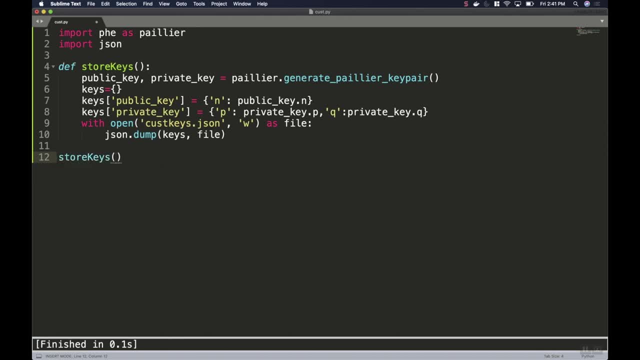 ahead and run this function so that I can generate my keys and store my keys as well. So let's go ahead and do that now. All right, Once that's done, let's get rid of this. Now I'm going to create a. 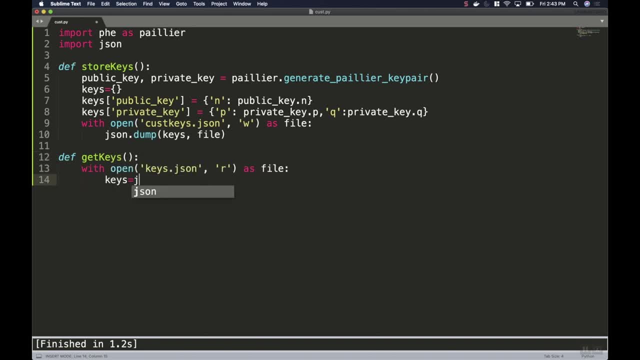 method that's going to allow me to retrieve those keys whenever I need them. So I'm going to go ahead and do that. Notice you'll see, this is keysjson. It should say cust keysjson. So this is an error that gets corrected later on. But it allows me to go ahead and pull my public key and 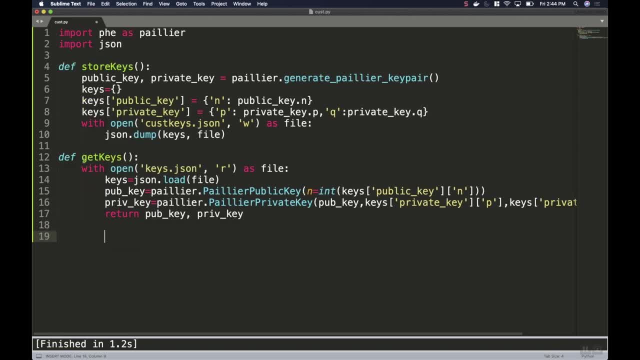 my private key as well. So just make sure you make that change and returns your public and private key. And next I'm going to go ahead and create a serialized data function, And this is going to take a public key as well as the data that I'm going to pass through later on. This is what we're. 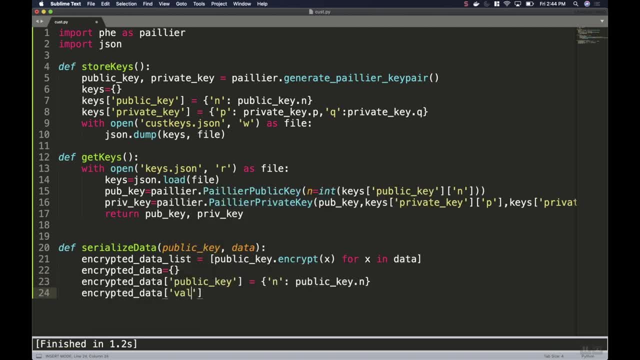 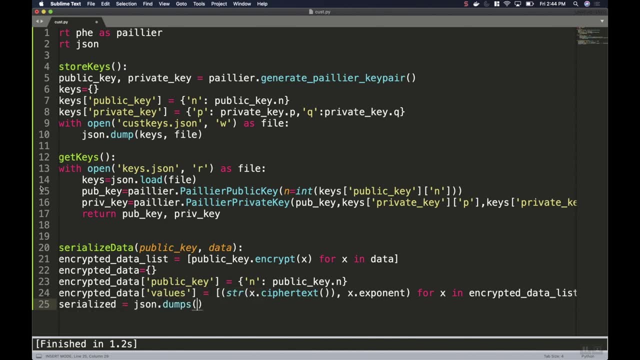 going to be passing on to the company in this case. So I'm going to be encrypting this data with my public key And I'm going to be passing in my public key, as well as all the values, as a ciphertext and an exponent. Then I'm going to go ahead and dump that as a JSON and send that back. Now it 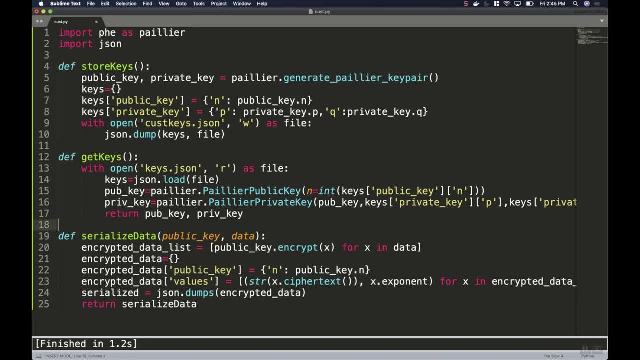 says return serialized data. Again, this is an error, Apologize for that. This should say return serialized, which is also corrected as well. All right, Next, let's start creating some data for this. Let's go ahead and get our keys from our get keys method that we created, The data that we're 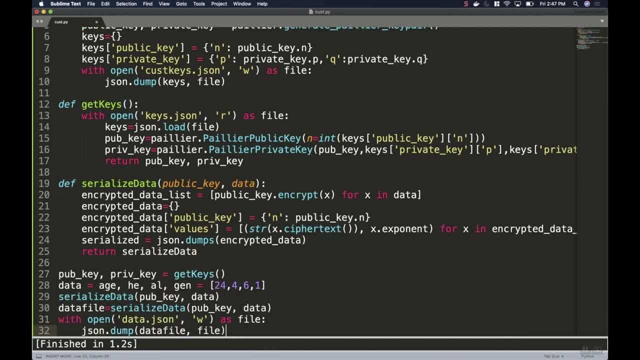 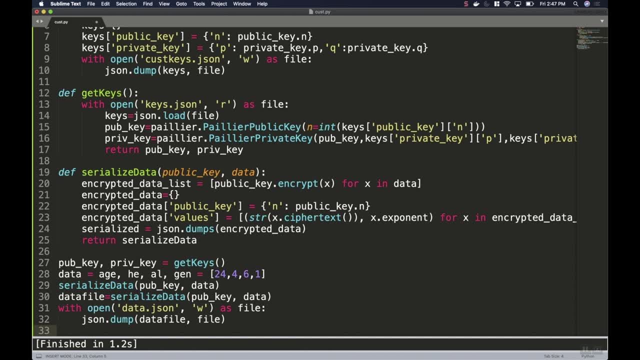 going to be passing on to the company corresponds to their age, their condition and whether they're male or female. We're going to serialize that data. I'm going to store it as a public key, passing the data with it as well, And then go ahead and save that as datajson And datajson. 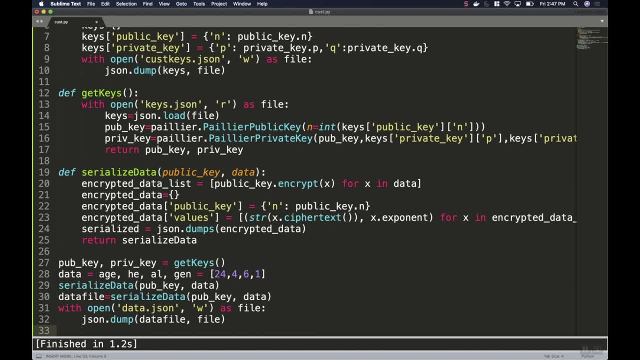 is what's going to go to the company in this case, And again completely encrypted. So we don't have access to this data. I don't know what's sitting in it. I'll show you in a very quick second that the data is, in fact, completely encrypted. So what I want to do is I'm going to go ahead and open up. 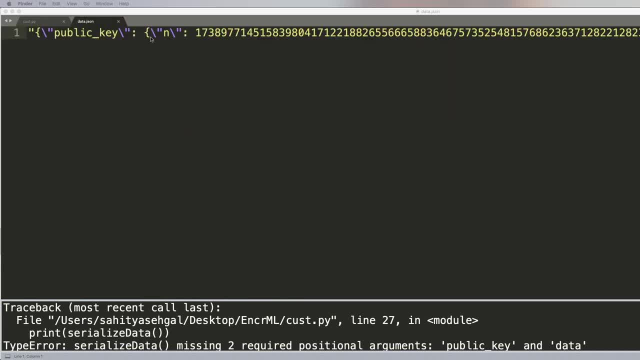 datajson, You'll see this is exactly what the company is getting, So there's no way for them to know what's in this. So this is the public key itself. As I scroll across, even the data here which is embedded in this variable called values, everything here is encrypted, So all these digits, 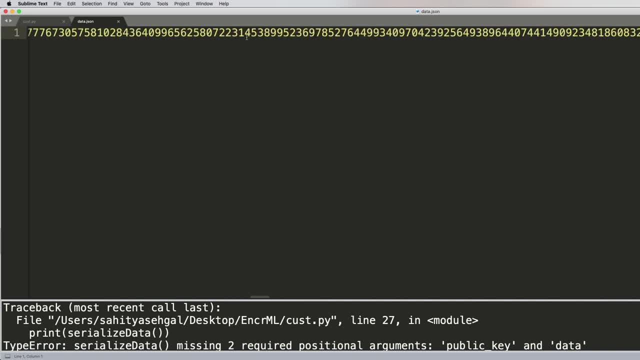 here is representative of that single digit, 24.. And then, wherever the next list element starts, which is right here, this is representative of that four. Only I know that because I'm watching it. There's no way anybody else will actually know what all this means. So this is what goes to the 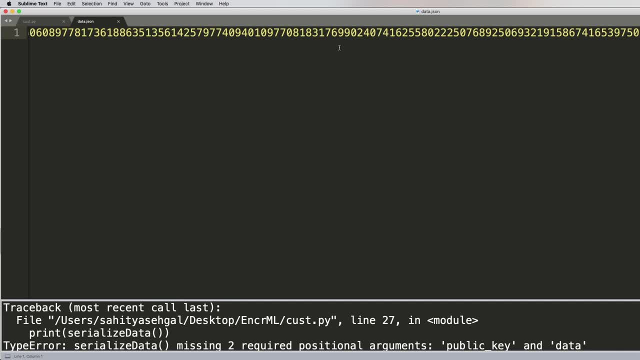 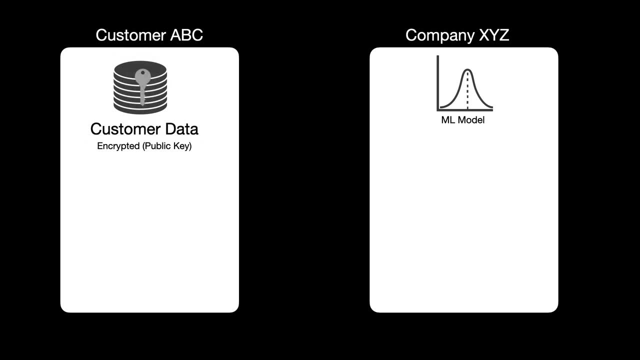 company, And the company is going to have to use their machine learning scalars against this to actually go ahead and build a model. So if we go back to our little example here now, we've encrypted the customer's data, which is datajson, And datajson is essentially what gets sent to. 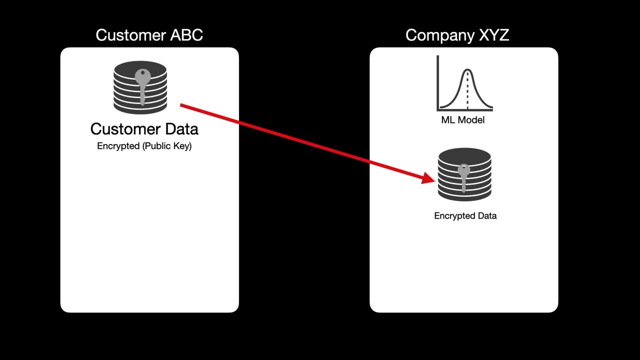 company XYZ in this case. So we've gone ahead and done that, And that's what the serialization piece does. So now the next thing we need to go and figure out is: okay, well, how am I going to be able to use this data And how am I going to be able to use this data? 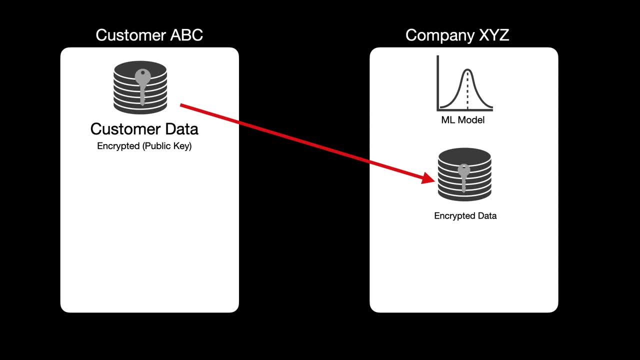 How am I going to take this data? How am I going to deserialize it so that I can actually use it in mathematical computations and then apply my model against it to come up with some kind of an answer, which is going to be my encrypted result. So we're going to do that next. So now I'm going. 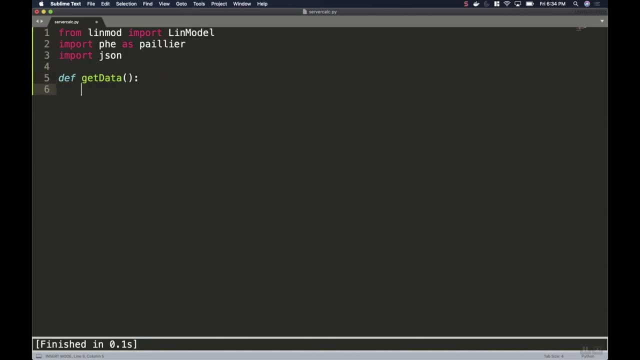 to create another file here called server calc, which is going to basically be my calculator on my server side under company XYZ. I'm going to go ahead and load some dependencies and go and get that jsondata that they sent me. Now I'm going to open it up. 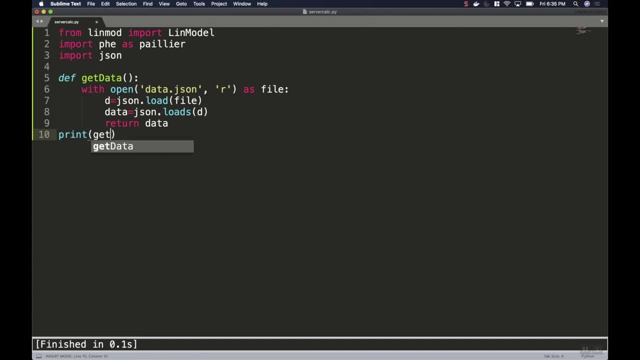 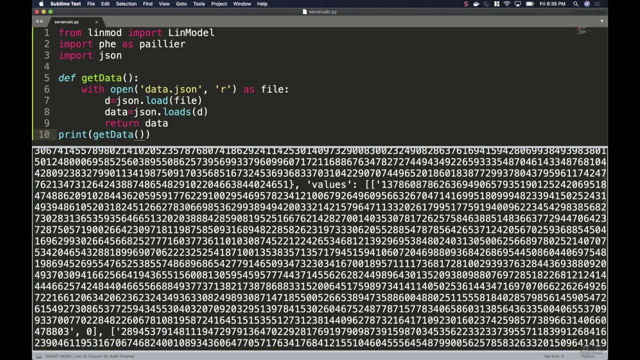 Here as well. So this is what the company XYZ would see when they go ahead and print, get data. So it's no different than what we saw in the json datajson file. Again, they're seeing a whole bunch of gibberish. This is completely encrypted data, So there's no way for them to decode this or make. 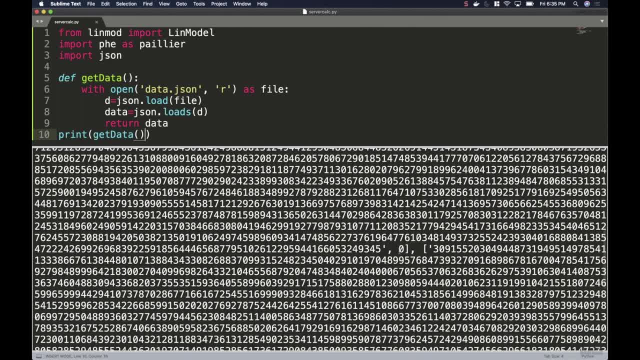 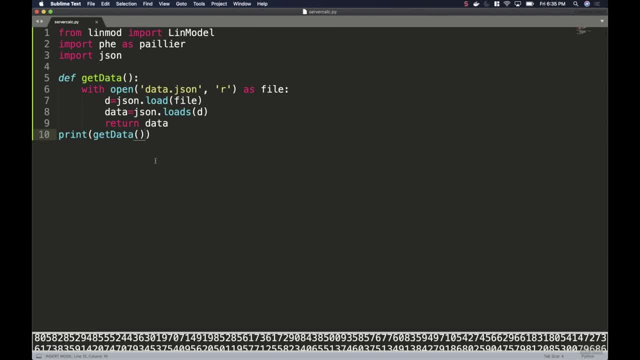 sense of this, because they don't have the private key that sits with the client And only the client can go ahead and decrypt this. So now the question is: how do we go ahead and build some kind of a model against this? So next, I'm going to be building a model against this. 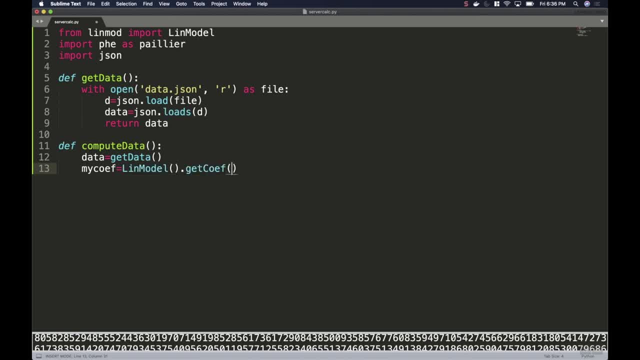 I'm going to be building something called compute data. What compute data is it's going to do is going to take the data that we have and it's going to take these scalars that we calculated in our linear model regression, which is what the my co-if in this case stands for. I'm going to. 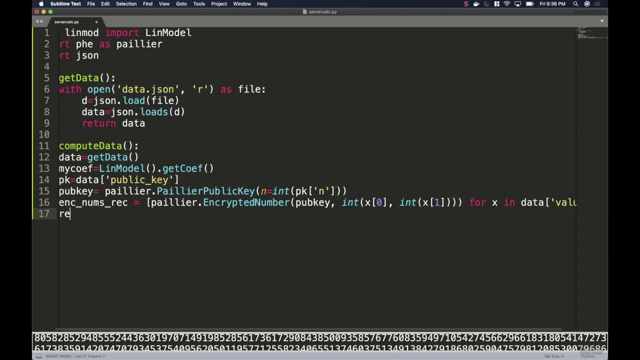 extract the public key from the data that I got- because, remember, the public key is a part of it- Then I'm going to go ahead and get that public key and make it usable so that I can encrypt these numbers in a way that I can deserialize it and then use it in my calculations. 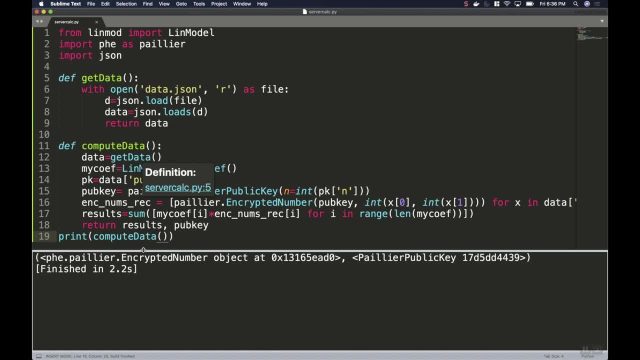 What I've done is I've taken the public key and I've taken the public key and I've taken the public key and I've taken those scalars and I've multiplied each scaler by each encrypted element in the list And I get an encrypted number object and then my public key in this case, which is what I'm. 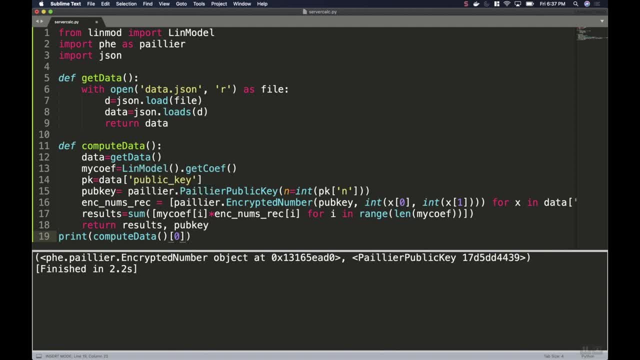 returning. So now let's go ahead and get the ciphertext of the actual results that we generated, in which case it should be just a one by one vector, because there's going to be no other list elements in this, because I've multiplied and added everything together, So this is the answer. 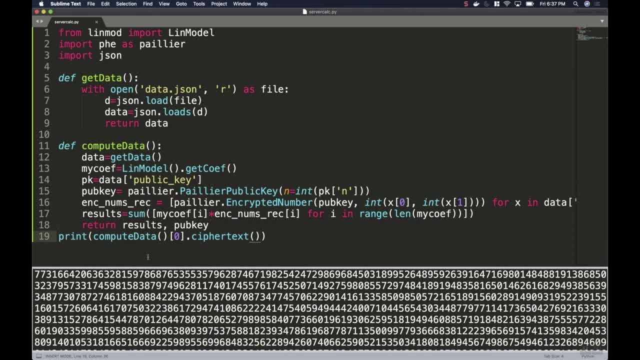 Now there's no way for me to know what this is, but I'm going to go ahead and do that. This is what I'm going to be sending back to the actual client for them to use their private key to decrypt against, And it should give me the answer using that regression model. All right, now that. 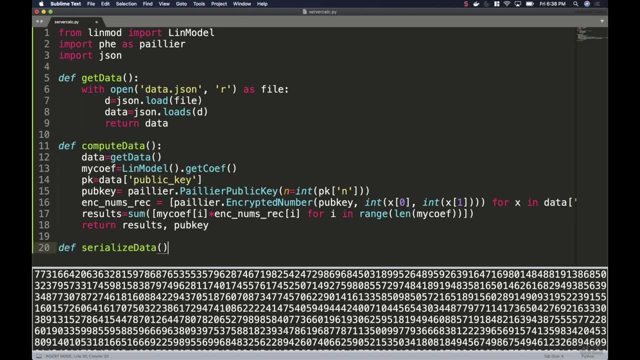 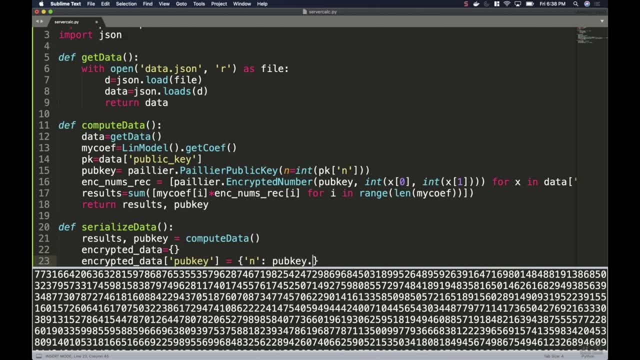 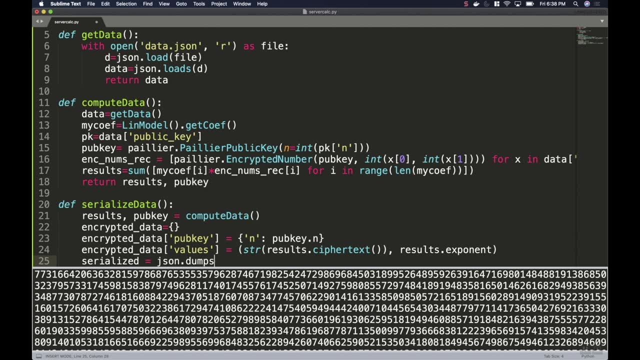 I've generated some kind of an answer. the next thing I need to do is again have a serialize data function again which is now going to send the encrypted result back to the client, in this case customer ABC. So I'm going ahead and I'm packaging up the public key again, And now the 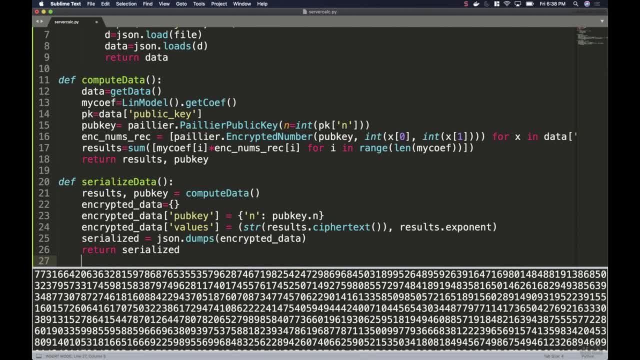 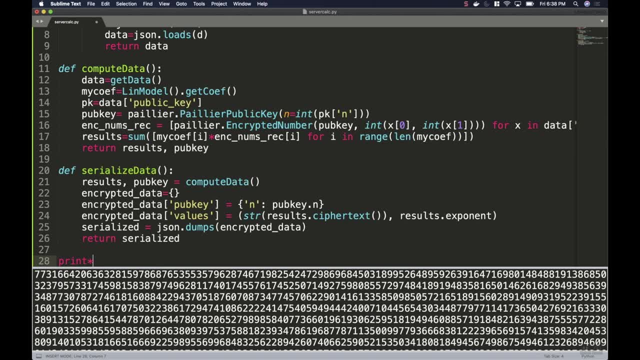 actual result. I'm actually going to go ahead and print this serialized result And you're going to see that again, it is completely encrypted. So this is the information that goes back, So it's a public key. the value, and then 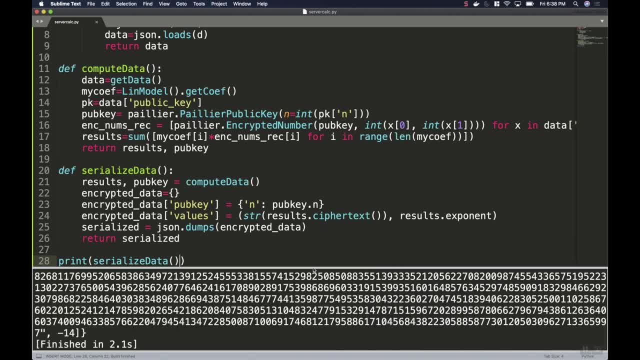 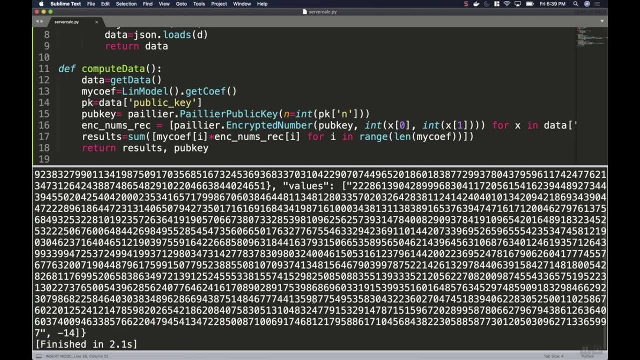 below you'll see there's an exponent of minus 14.. This goes back to the client, and they have to now use their private key to decrypt, whatever this means. At this point, company XYZ will have no further ability to decrypt anything, So we're going to go ahead and print the serialized result, and this is the actual. 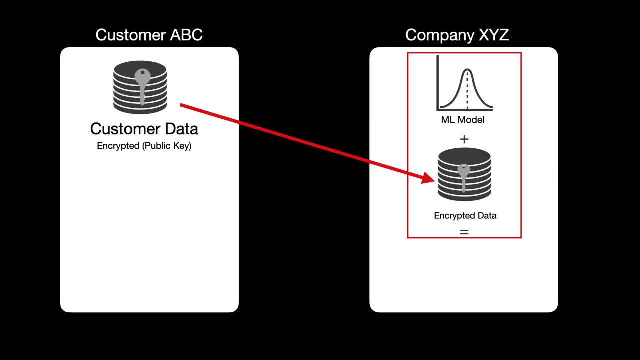 to decrypt this now. all right. so, going back to this example, what we've done is we've taken the ml model, we've taken the encrypted data and we've gone ahead and created the encrypted result, which is what you just saw. right now, what we're doing, then, is we've packaged this up as a json. the next, 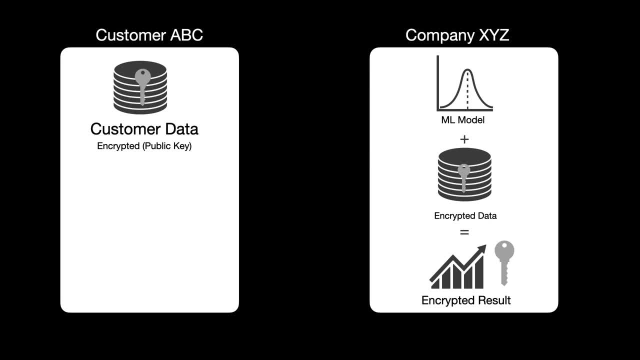 step you're going to see is we're actually going to go ahead and send this back to the customer in the form of answerjson. so we're just going to go ahead and create a very small little function or a little snippet of code that's going to allow us to take that serialized data now with the 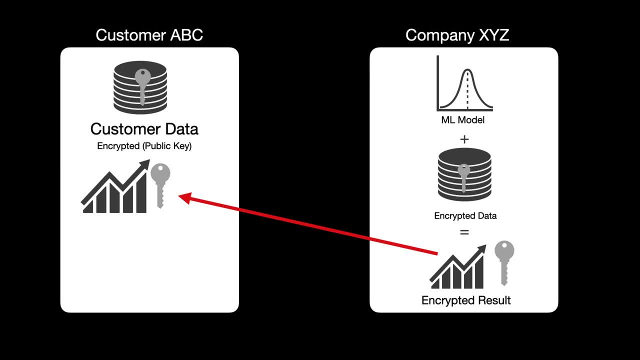 encrypted result that you saw that had the public key, the encrypted values themselves and then the exponent, and that's going to go back to the customer as answerjson. so let's go ahead and see what that looks like. all right, so now you're going to go see that i'm building the main function. 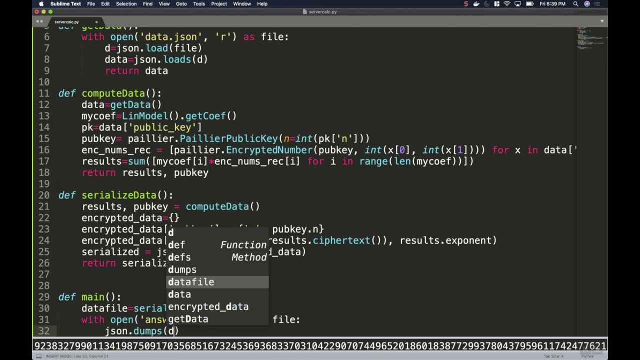 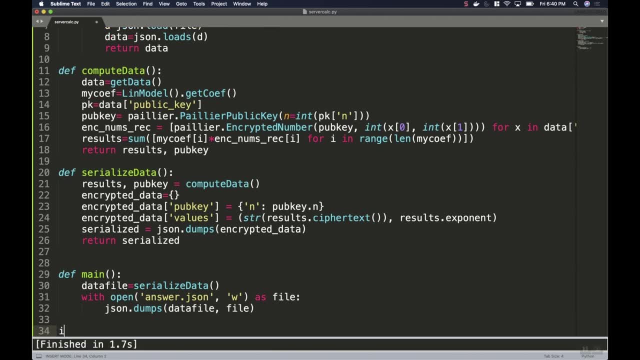 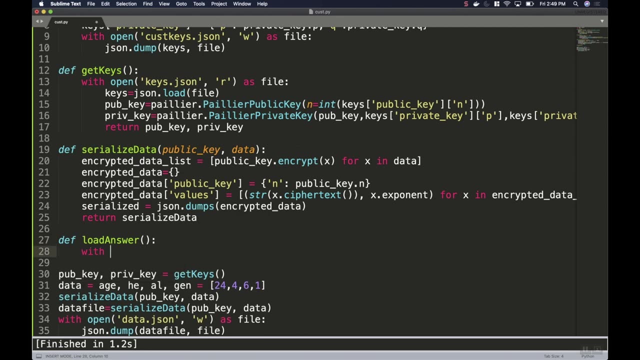 here i'm going to set my data file equal to my serialized data, again using the with open answerjson, and writing it to a data file called answerjson, and then just closing it out with my if name equals main function. all right, so we're back in the customer file now. so now that the customer has got access, 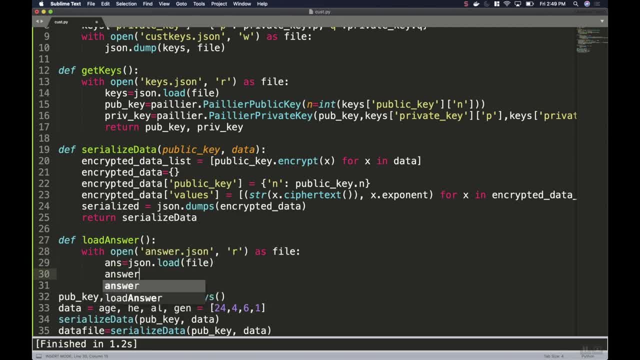 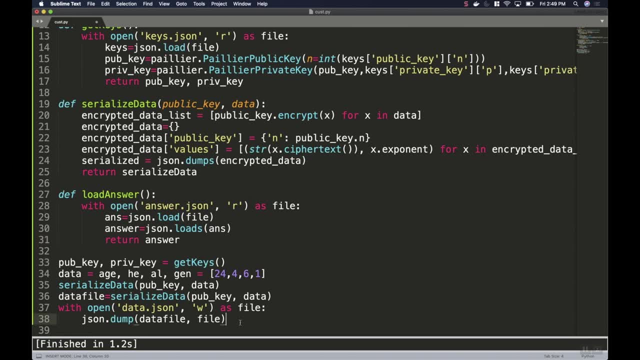 to that answersjson data now they're going to. now we're going to build a function that's going to allow them to unload that data now. so i'm basically loading that data, calling it answer and returning answer back. now i need to build another function which is going to allow me to. 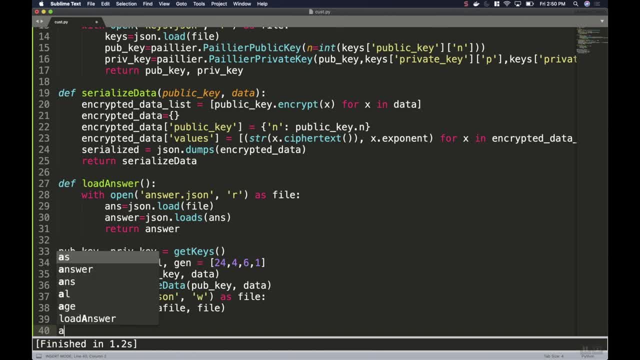 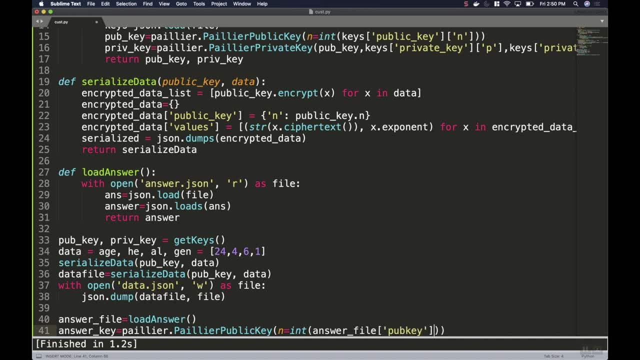 take the answer file, load it, and now i'm going to be able to go back to the answerjson and load it back into the answerjson. and load it back into the answerjson and pull my public key out of this and then pull the encrypted number from this as well using the. 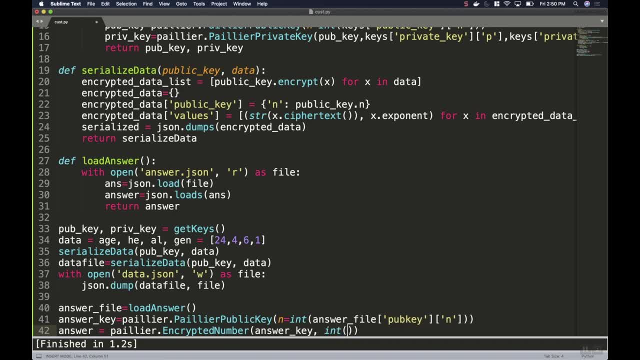 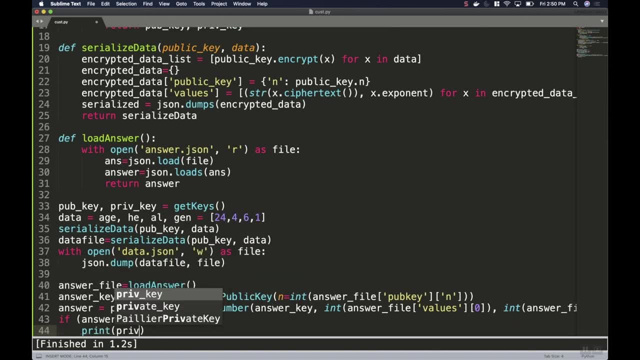 you know, public key, the, the ciphertext and the exponent. and if the public key that i get back from the file that the company sent me matches the public key that i have, then i'm going to use that private key to go ahead and decrypt the information. all right, so? and if this checks out, 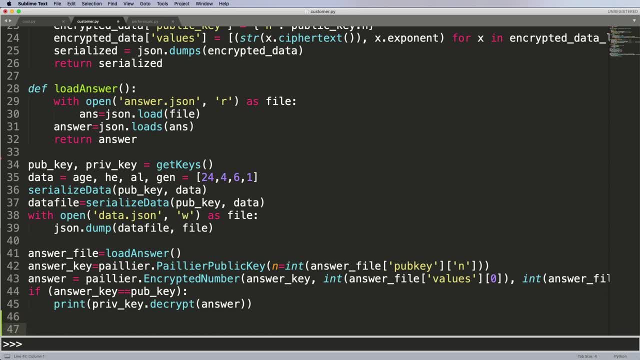 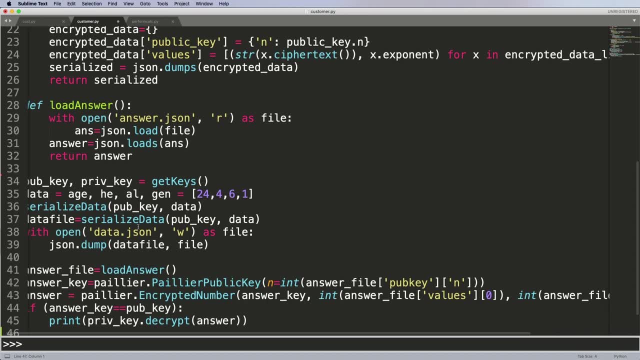 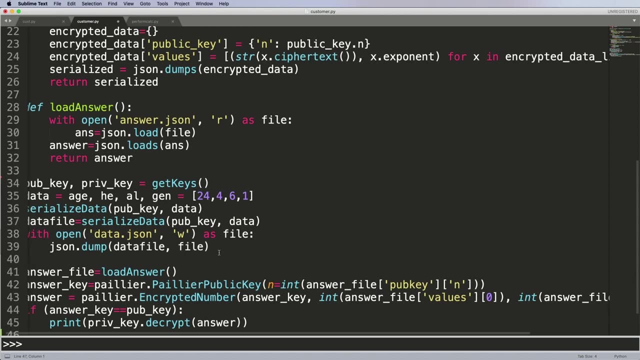 then we're going to go ahead and print our answer for this regression model. so before we do print it again, remember this was the original data, the 2461. i don't have the scalars here that were from the machine learning model because i came from the organization or the company that i sent my data to. i got back an answer and now i'm going. 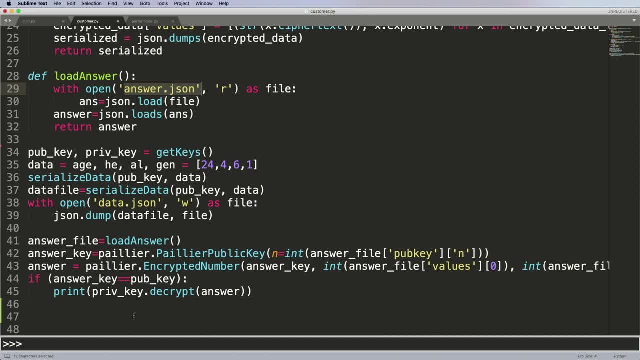 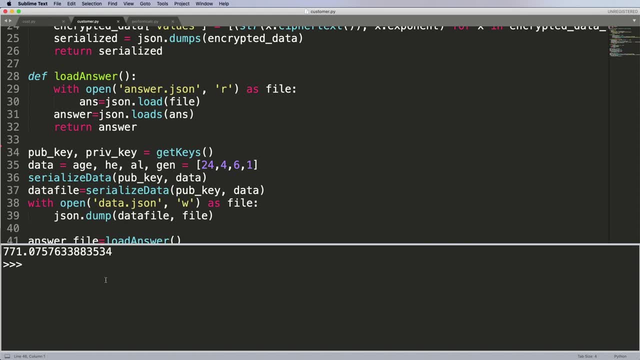 to go ahead and see whether this answer or not is going to give me some kind of a result. so let's go ahead and run this and pull this up, and the answer i get back is 771. now that doesn't seem out of line when we look at some of these numbers here. i mean, you know, we do have numbers that are in the 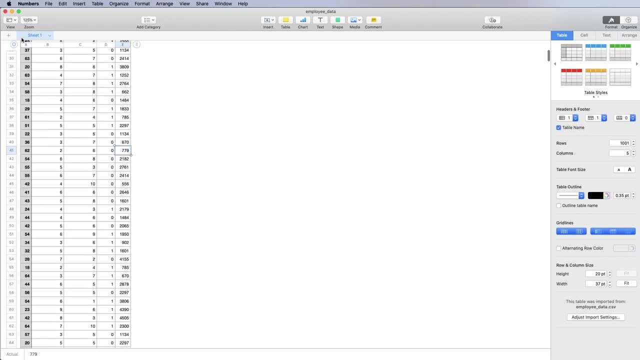 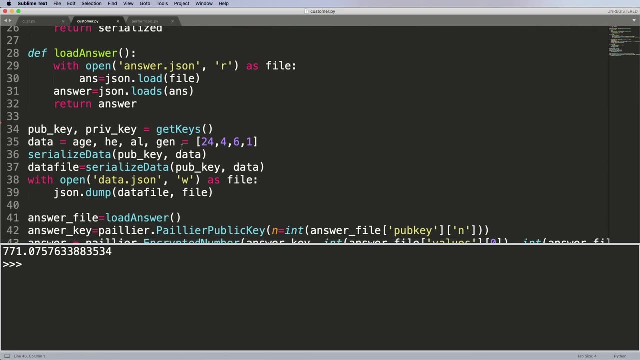 right order, um and so forth, so 779, so nothing. that is, uh shocking when i look at it. i think what i want to figure out now is, now that i do have access to those scalars. so let's say, this was the data that i'm looking at. i actually want to test whether or not the encrypted data did the. 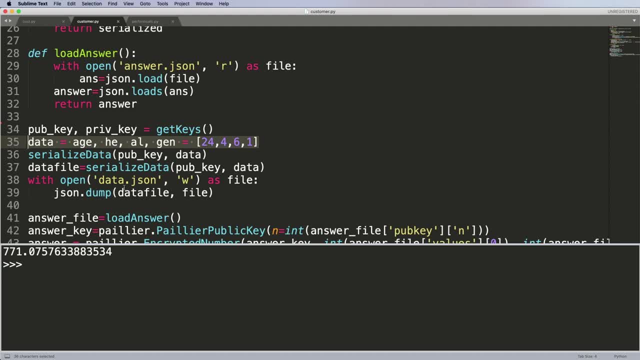 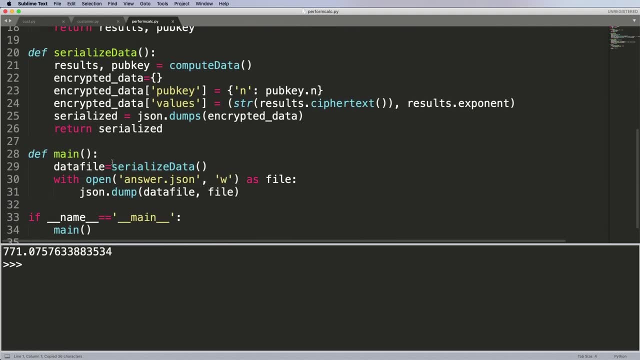 calculations properly. so 771 is what this gave me. when i use this encryption method, let's just go ahead and let's go back to this file here, where we know that this is sitting on the company's server, and again remember, when the data is encrypted, it's not going to be the same as the data that 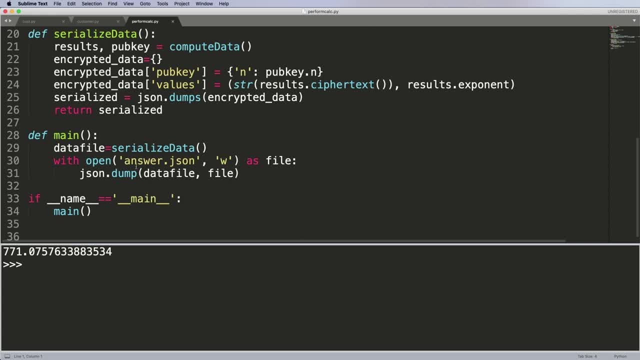 the company got these scalars, they were encrypted, so i'm just going to go ahead and drop these actual data values in here, so we know that data has these specific numbers. i know i have access to my coefficients here through the linear model in theory, if i were to go ahead and calculate. 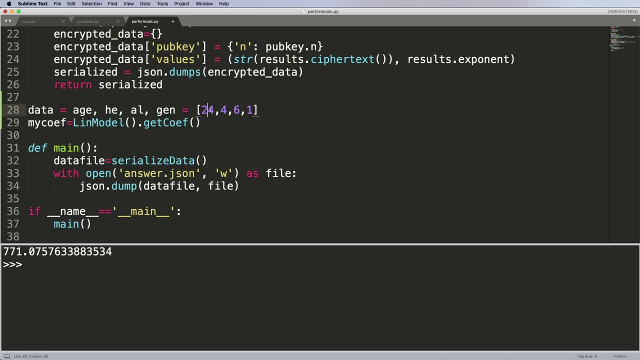 the coefficients in this linear model. with these numbers, i should get that same number, 771. so let's go ahead and give this a shot. so i'm going to type in print and we're going to go ahead and sum everything up and we're going to sum up a list. so this is going to be a list of lists, basically. 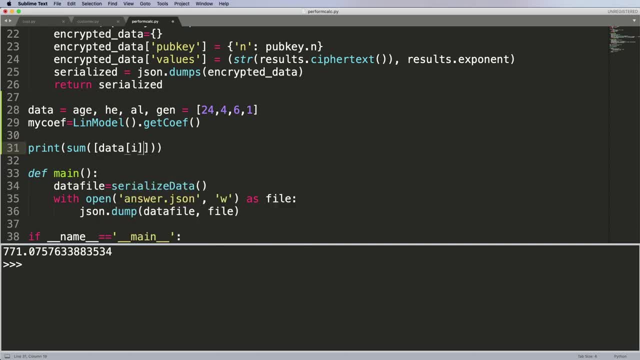 or a list of elements. so data: i times my co fi for i in range len data. so basically it's: it's taking the first element in here multiplying by 24, the second element multiplying it by four and so forth, and we should get this number here as well: 771. so let's go ahead and do that, and we're going to go ahead and do that. 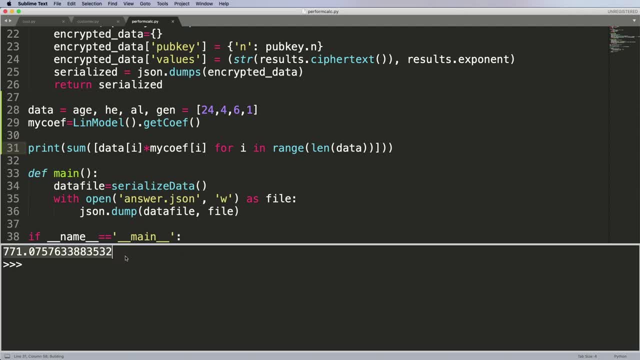 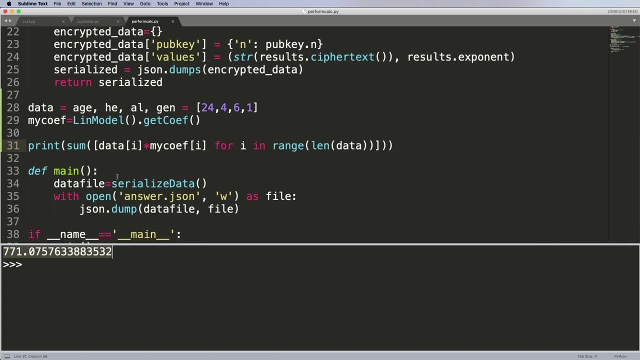 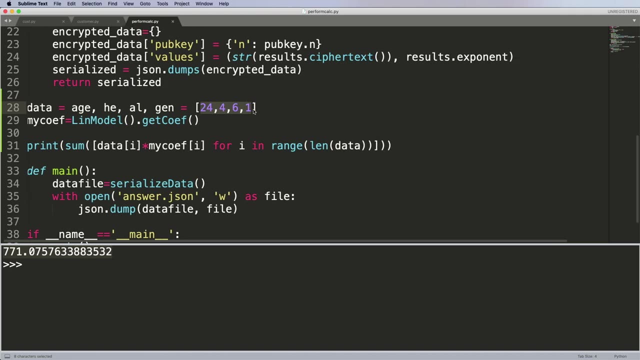 if i hit print, i get 771, so what that tells me is that it's actually done the calculation correctly. so, in essence, what we've been able to successfully do is send this data in an encrypted format to an organization, because we don't want them to know these numbers. they took encrypted data. they did. 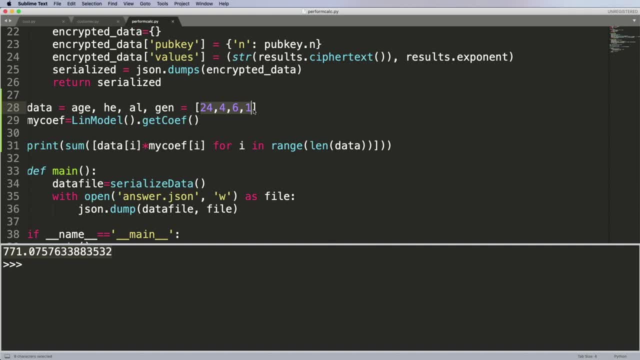 machine learning against it. in this case, a linear regression model sent back an encrypted result. we decrypted that with our private key and we got an answer, which is kind of cool. so this actually works really, really well. all right, so let's take it from here and review what happened. so company xyz produced answerjson. 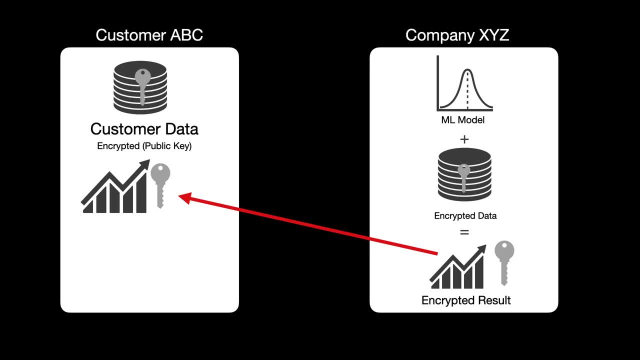 they went ahead and they sent answerjson to customer abc. customer abc then compared the public key that was sent by company xyz to make sure nothing was changed or modified or the wrong file sent. compared it to the public key that they had and, if they matched, use that private key to. 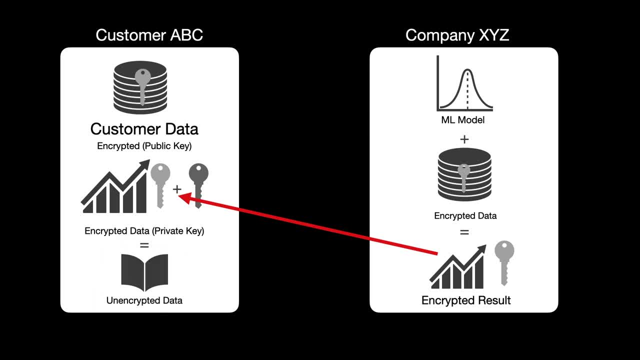 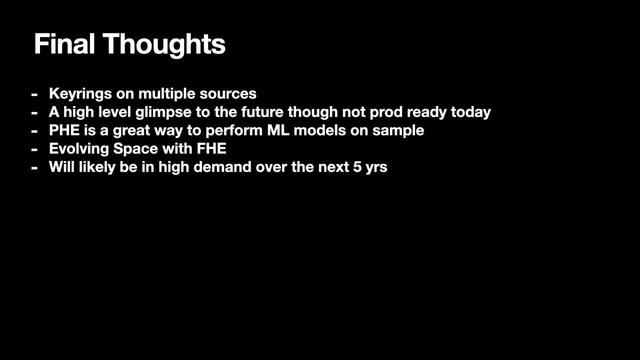 go ahead and encrypt that data, and then finally came up with the encrypted data, unencrypted data, which in this case was 771. all right, so let me just share a couple of final thoughts on this. first of all, you know, just in terms of some of the concepts with phe or partial 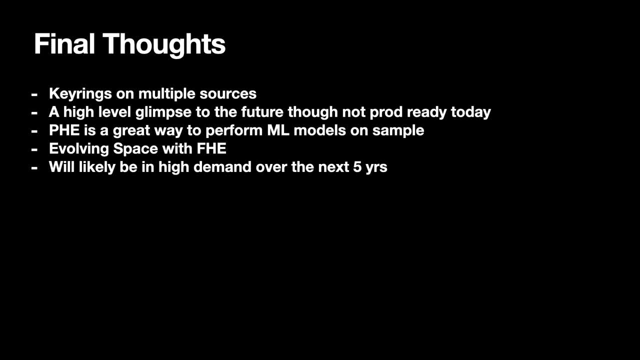 homomorphic encryption. we didn't get into the concept of key rings. key rings are basically a way for you to store multiple public and private keys. so, for example, if i had customer abc but i had company xyz and company def, i have the ability to just put all my keys in one key ring. 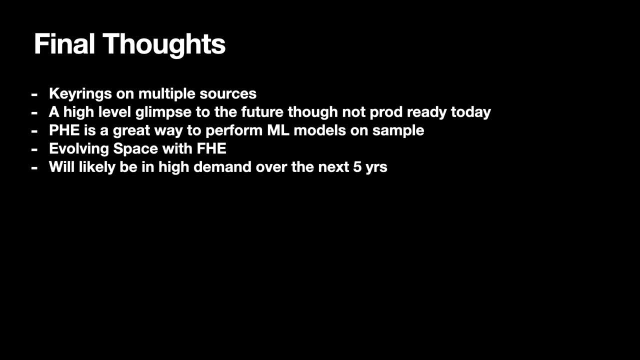 and i can go back and search for that key ring based on the public key, so it just becomes a lot easier. i don't have to worry about managing multiple keys, so that's something that is available in the docs for you to look at. i've tried it myself. it's actually pretty cool. i just 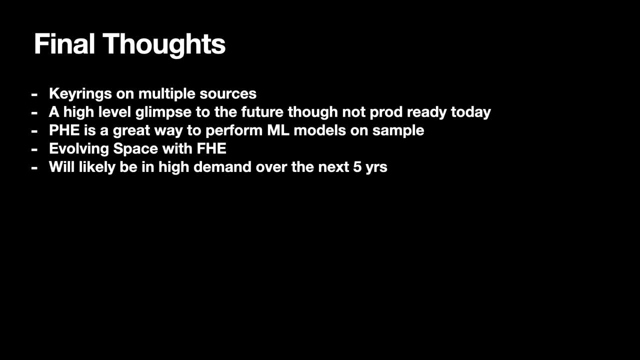 didn't want to go over it today because i thought it'd be a little bit overload with the subject. the second thing is: you know this is a glimpse into the future, though i would say it's not production ready at this point. i'm not aware of anybody who's actually put it into production. 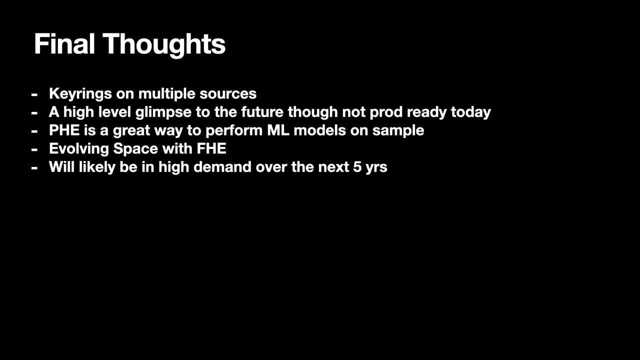 right now it seems like it's really heavy on the research side of things, so i'm not sure if it's going to be a huge market for this in the future. if you wanted to go ahead and just explore some basic algorithms, i think this is a great way to do it. uh, today, just to sort of play around with it. 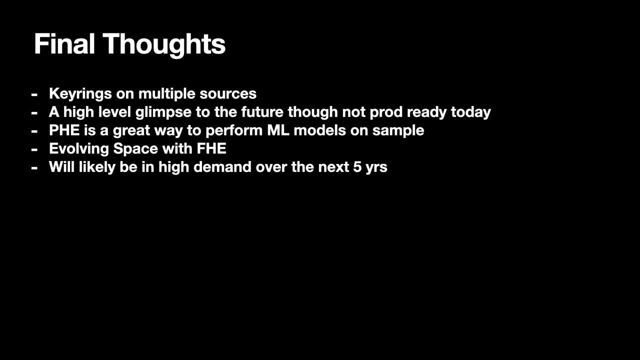 but even just start learning and understanding a little bit about how data encryption works. you know whether you're looking at database encryption or whether you're looking at data encryption- the way data travels. there's a lot of value in understanding how you can do that, especially as privacy becomes more and more important, and i think it's a great way to. 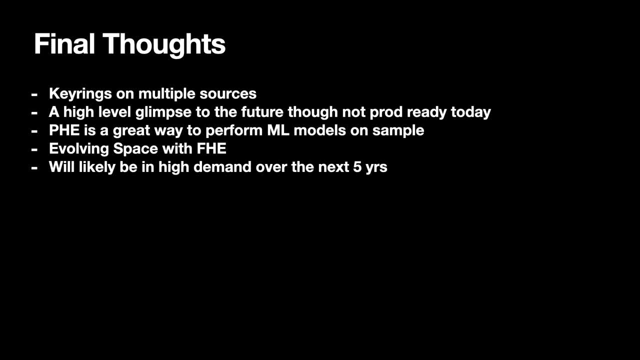 keep yourself on top of mind with some of these organizations out there. again, like i said, it's an evolving space and with things like fully homomorphic encryption out there, there's so many more possibilities you can do, so you can get into more of the complex modeling. i've seen some 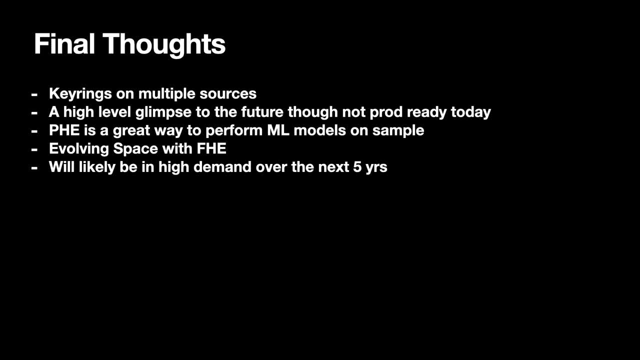 research papers that actually have neural networks built off of fe, which is kind of cool and it has a lot more intensity, and, as well, things like bootstrapping, slash padding, which is basically a way to add- you know, we'll say noise- into your encryption model, so that 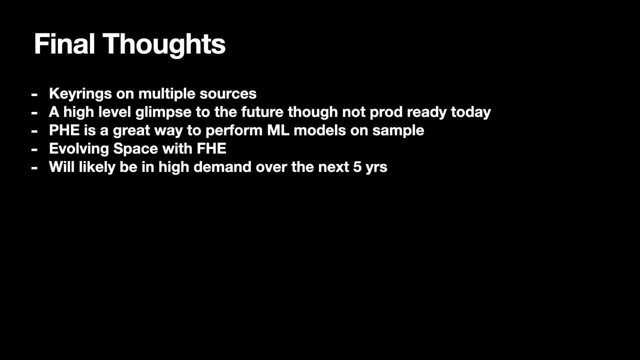 it's not easily something that you can go back and break or figure out. So there's a lot of cool things happening in this space And my prediction is there's going to be a high demand for this over the next five years, Like I said, as privacy becomes more and more important to people. 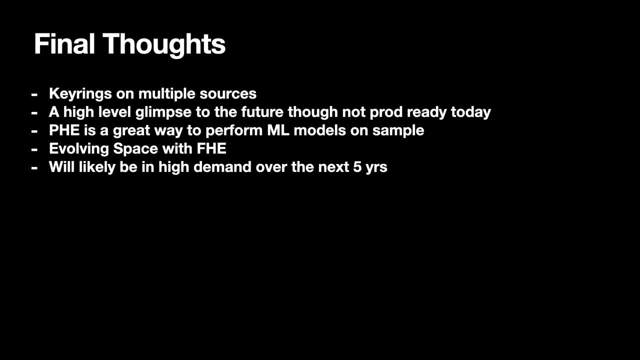 and there's more organizations looking at it- a lot of investment going in this space, the ability to actually mine data. that's very private, especially with organizations- or even countries, for that matter- that have really tight regulations against how data sharing practices look like. 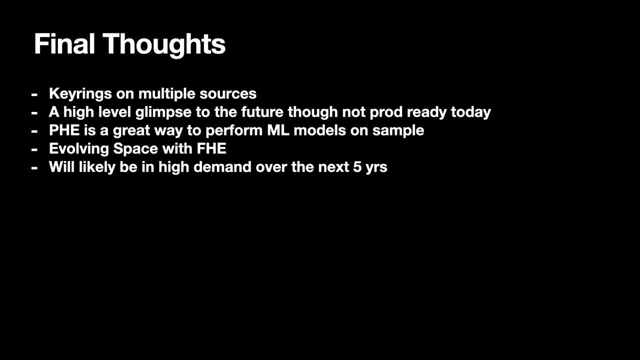 encrypting that data is a really good way to get around it but at the same time figure out how to mine it. But I don't think this is going to be production ready, probably for another two to three years. At least that's my best guess at this point.